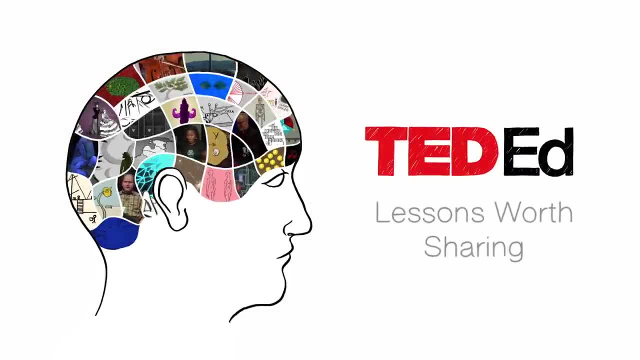 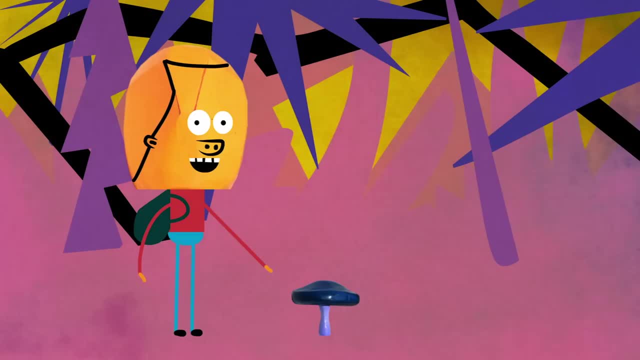 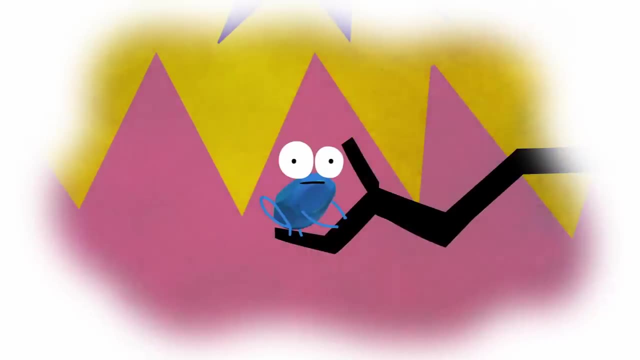 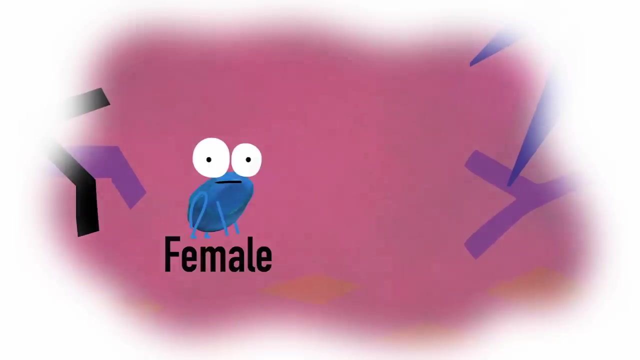 So you're stranded in a huge rainforest and you've eaten a poisonous mushroom. To save your life, you need the antidote excreted by a certain species of frog. Unfortunately, only the female of the species produces the antidote. And to make matters worse, the male and female occur in equal numbers. 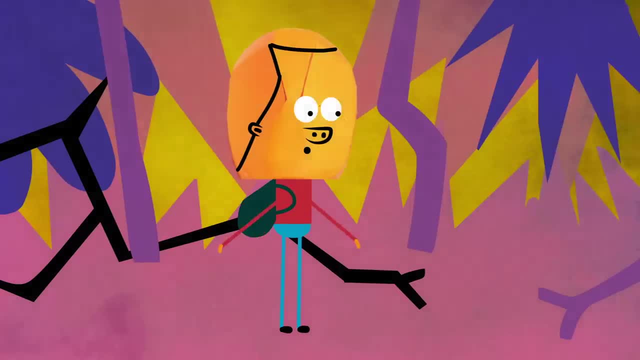 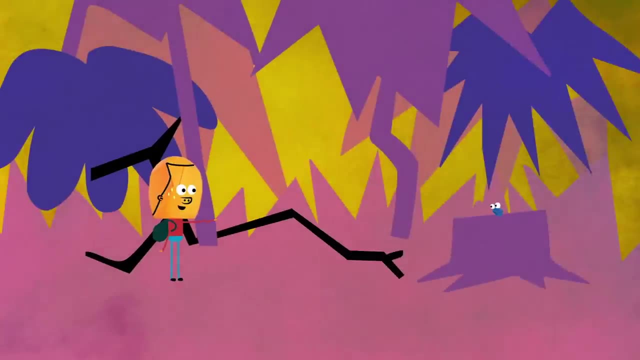 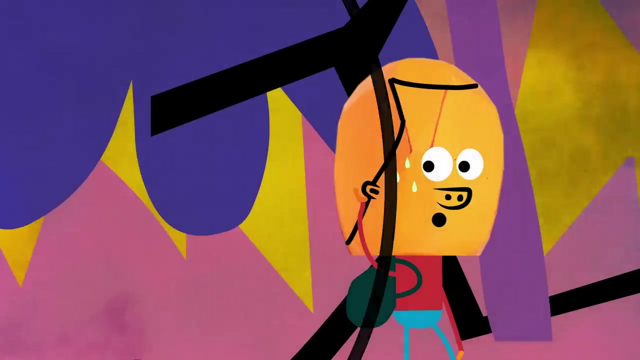 and look identical, with no way for you to tell them apart, except that the male has a distinctive croak. And it may just be your lucky day. To your left, you've spotted a frog on a tree stump, But before you start running to it, you're startled by the croak of a male frog. 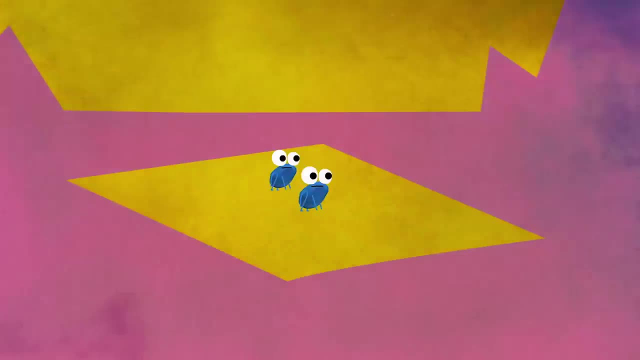 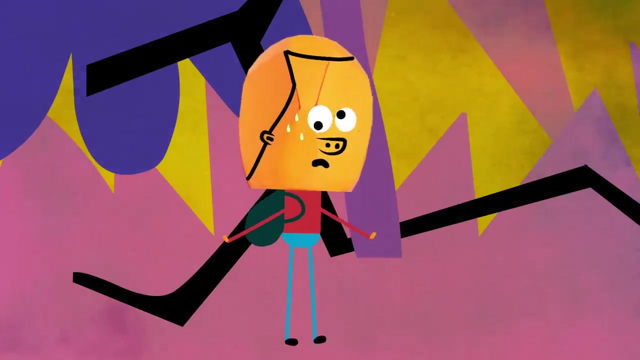 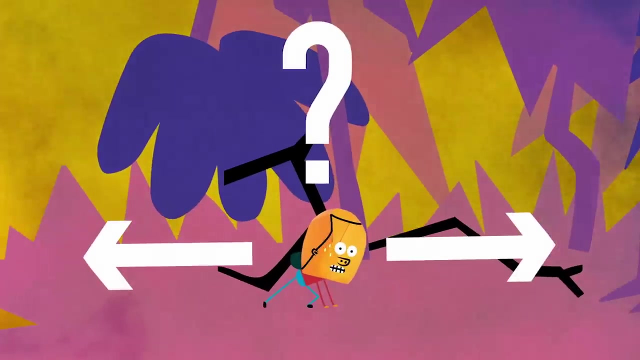 coming from a clearing in the opposite direction. There you see two frogs, but you can't tell which one made the sound. You feel yourself starting to lose consciousness and realize that you only have time to go in one direction before you collapse. What are your chances of survival if you head for the clearing? 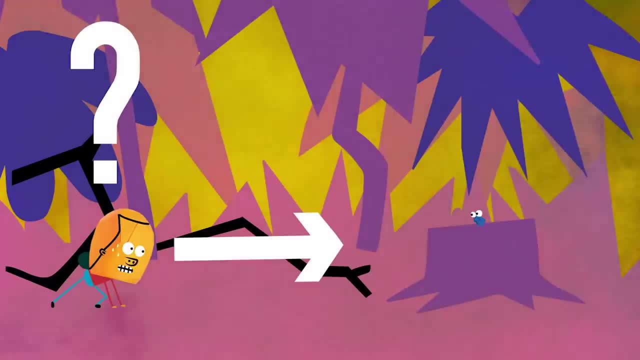 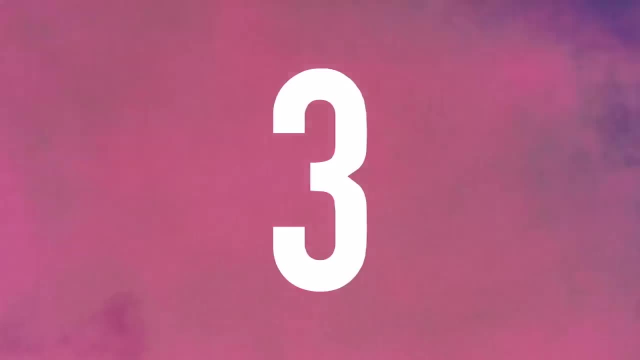 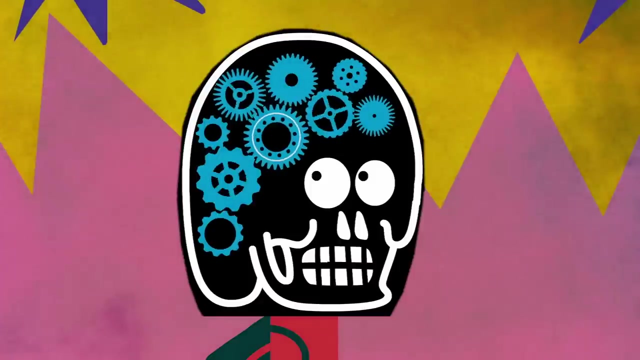 and lick both of the frogs there. What about if you go to the tree stump? Which way should you go? If you chose to go to the clearing, you're right, But the hard part is correctly calculating your odds. There are two common, incorrect ways of solving this problem. 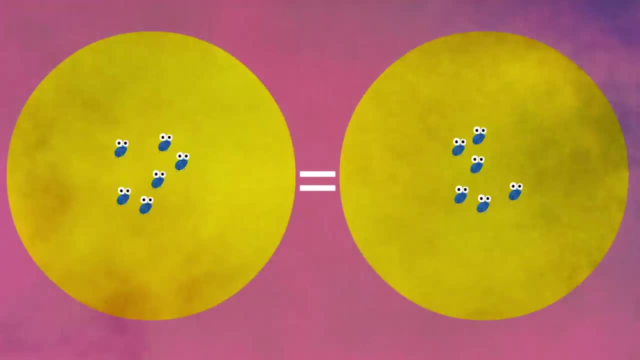 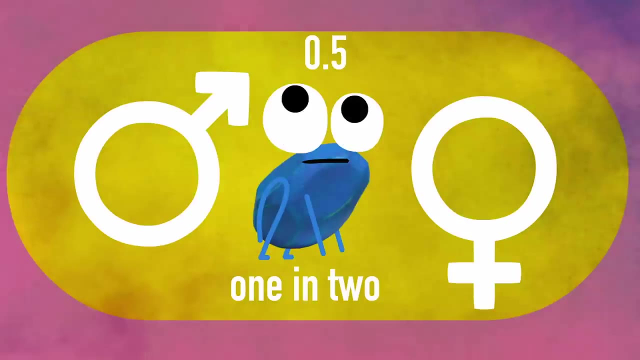 Wrong answer. number one: Assuming there's a roughly equal number of males and females, the probability of any one frog being either sex is one in two, which is 0.5 or 50%. And since all frogs are independent of each other, 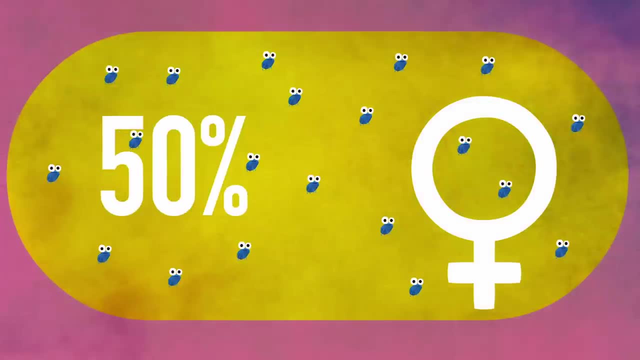 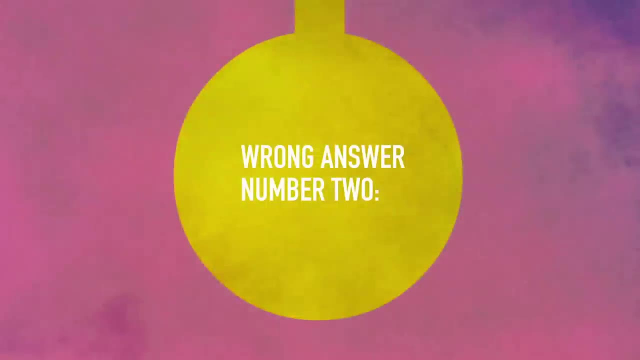 the chance of any one of them being female should still be 50% each time you choose. This logic actually is correct for the tree stump, but not for the clearing. Wrong answer two. First you saw two frogs in the clearing. Now you've learned that at least one of them is male. 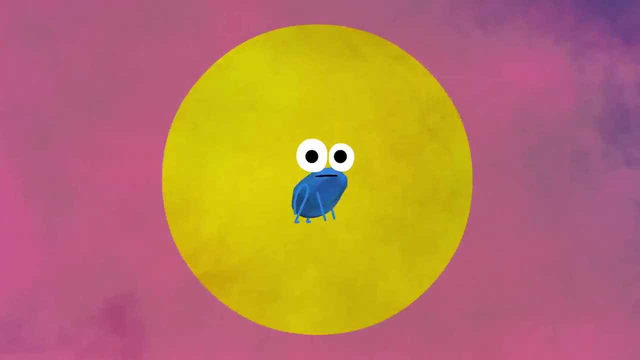 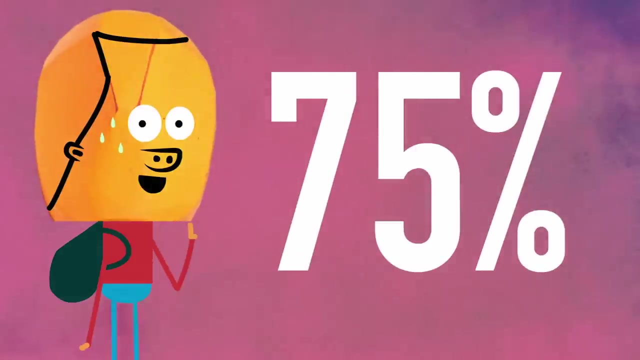 But what are the chances that both are? If the probability of each individual frog being male is 0.5, then multiplying the two together will give you 0.25, which is one in four or 25%. So you have a 75% chance of getting at least one female and receiving the antidote.